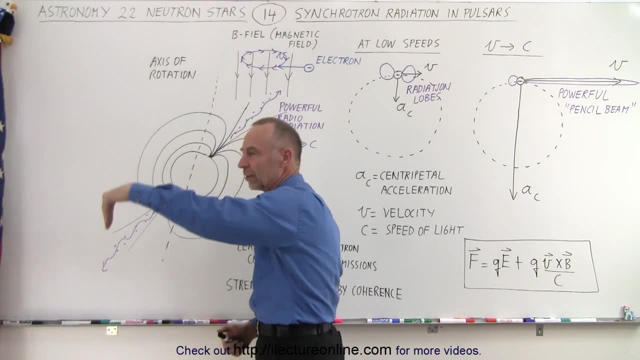 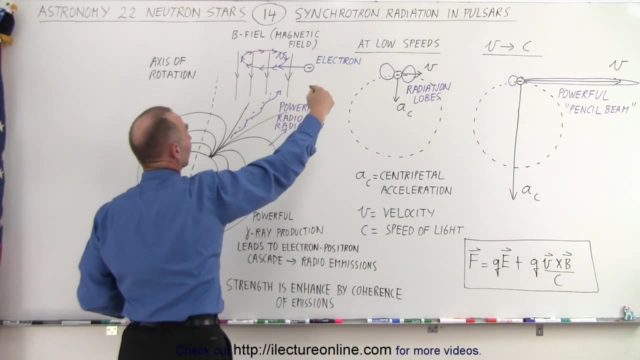 then you curl your fingers in the direction of the magnetic field and your thumb will point in the direction of the forces against the electric charge, in this case the electron. So it's feeling of force that's causing the electron to go around in circles, and so that's part of the driver of the synchrotron motion. 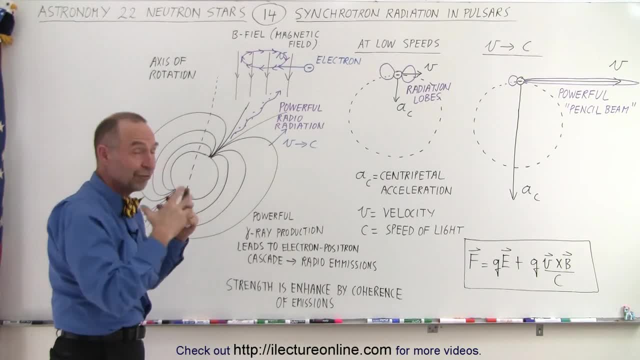 So when electrons come into contact with a very powerful magnetic field- and we saw in the previous video how powerful these magnetic fields are, how strong they are- then the electrons start zipping around in very tight circles at very high velocities And then it sets a very strong electric field that shoots the particles out in both directions. 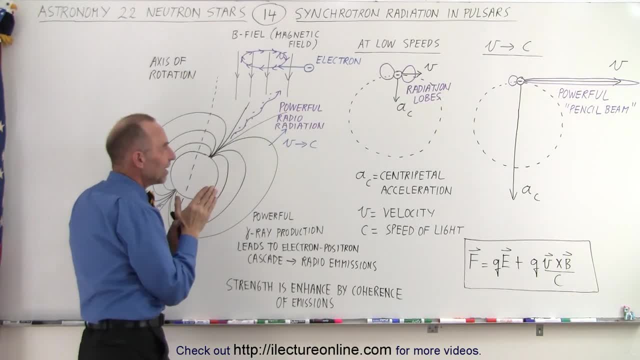 so they go spiraling upward at very high velocities, sending beams of radiation in that direction as well. In addition to that, we have the production of gamma rays. Now, very powerful gamma rays can be used to produce electrons and positrons. positrons are the antiparticle of the electron, and so we produce electron-positron pairs in a cascade format. 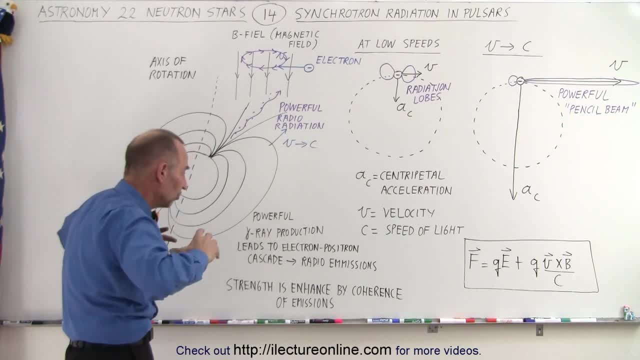 So, in other words, there are so many gamma rays produced that we produce an enormous amount of electrons and positrons and they go cascading out, causing the radio emissions. So, in other words, what we have observed if we see particles that move out along the direction of the magnetic field. 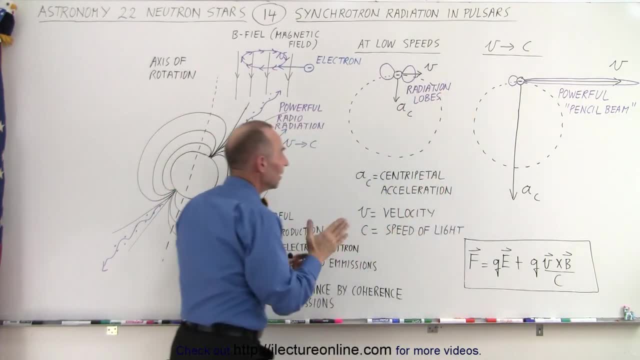 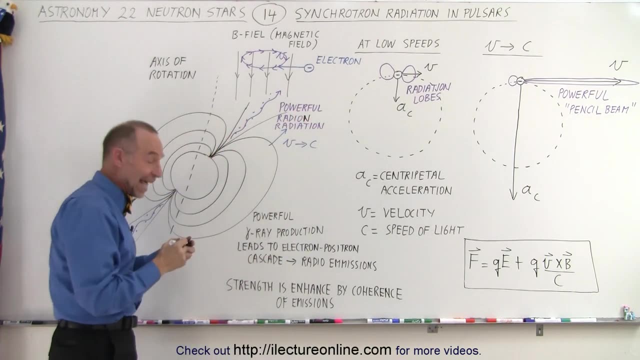 at enormous speeds, speeds reaching the speed of light, and therefore in the direction of that motion you get very powerful radiation- and I'm missing an N there on my radiation- and so that's how those radio signals are produced. Now, of course, since the neutron star is rotating about the axis of rotation, 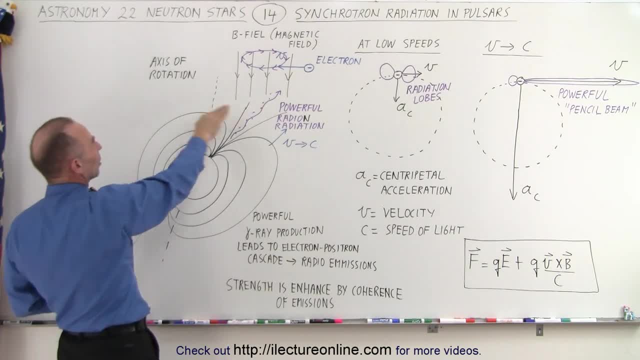 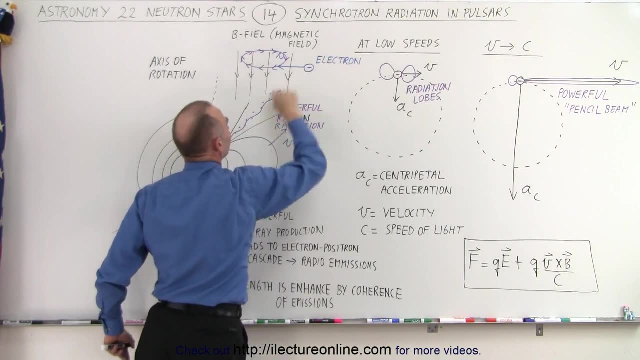 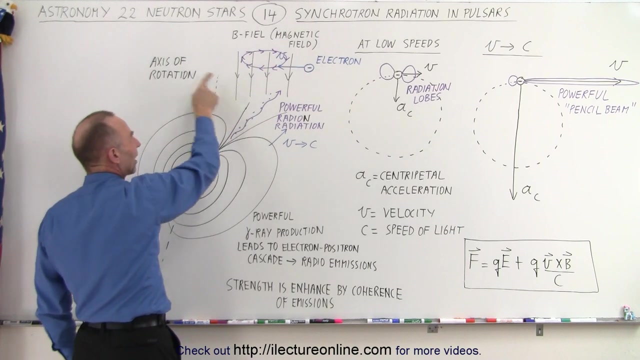 that beam then goes rotating around, kind of making a cone shape, and then if at one point in time the beam is pointed directly in the position where Earth is, then we see these flashes of electromagnetic radiation, radio radiation, every time the beam passes in that line of sight. 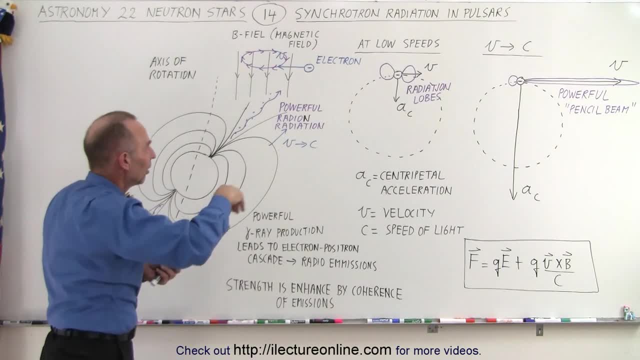 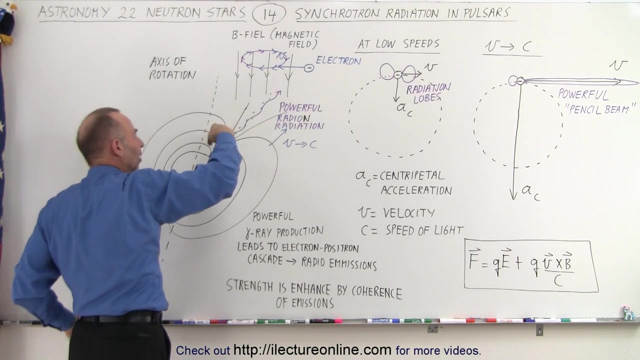 But it's the synchrotron motion caused by electrons being injected into the magnetic field to production of powerful gamma rays, then the cascading of electrons and positrons which then get pushed to very strong electric fields into both directions, opposite in direction, along the line of the magnetic fields. 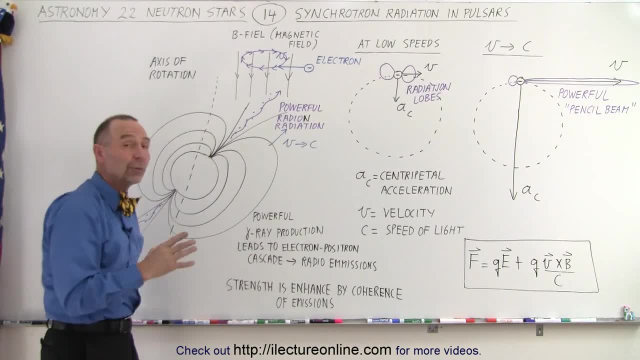 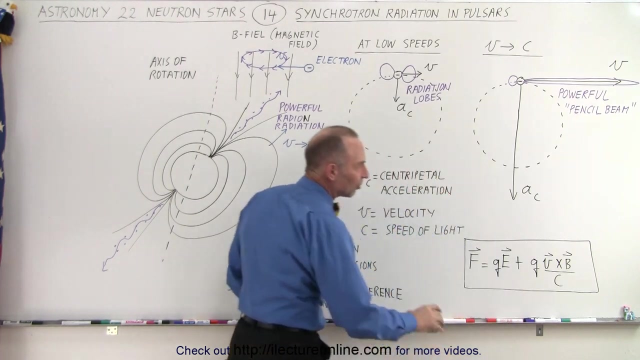 and that causes these very powerful radio radiation to be emitted in the direction of travel, based upon the synchrotron radiation principle. So the forces they feel is a combination of the electric field forces plus the combination of the magnetic field forces. The magnetic field forces cause it to rotate within the field. 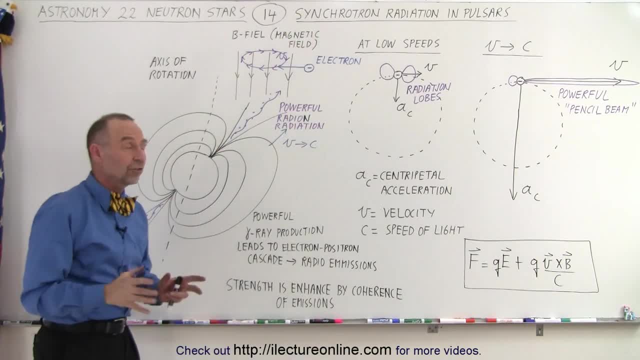 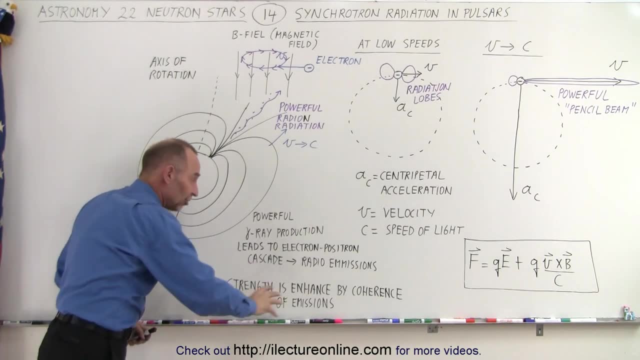 and the electric field accelerates it out in both directions, causing the radiation then to move or to go out in the direction of travel. It's complicated, It's modeled. These are theoretical models. Of course, we're not there taking close observations. 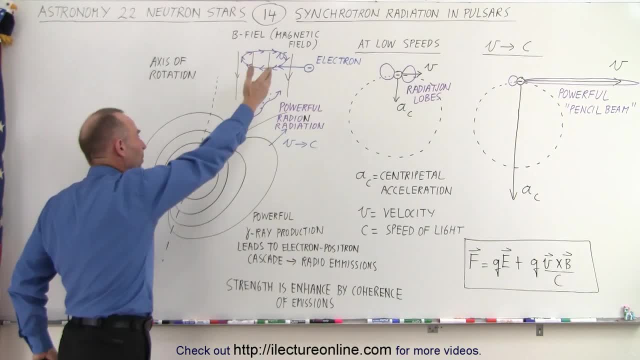 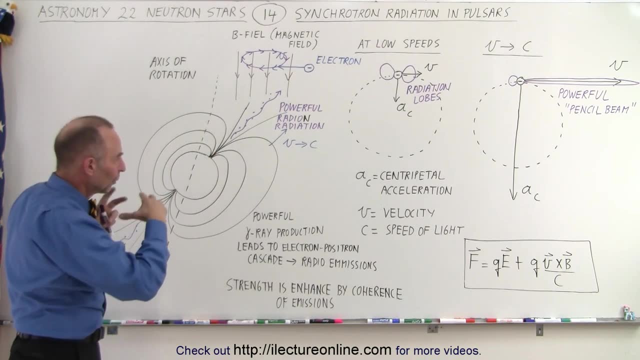 What we do see in the end that we see these charged particles moving in both directions at very high velocities, near the speed of light, any time we have a pulsar or we have other engines like black holes that shoot these particles out at very high velocities. 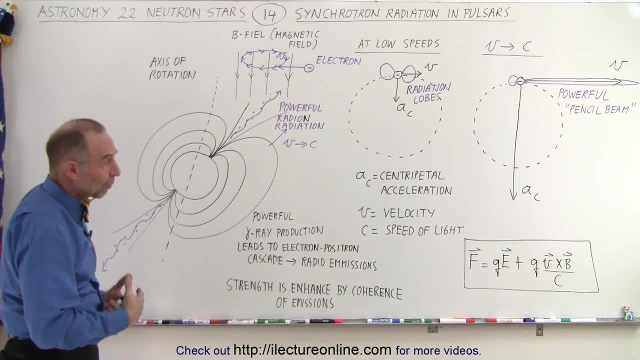 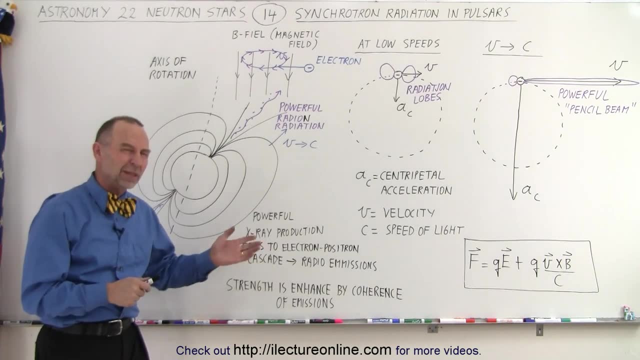 causing this kind of radiation to exist. So it's what we observe and it's what we model to try and explain the origin of that radiation. And that is pretty well the way we think, Of course, the way we theorize how everything happens. 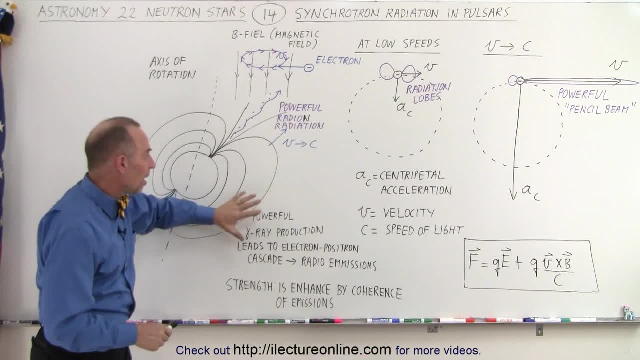 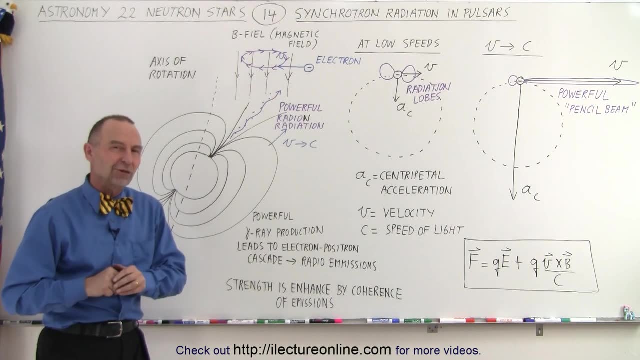 This we're positive of This. here is a theorized model that explains pretty well what we think is happening there, And that's the explanation we have for that powerful radio radiation coming from pulsars. So if it wasn't for the electron, you wouldn't see it. 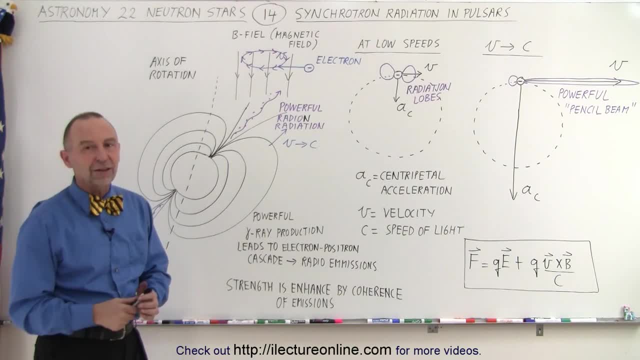 If it wasn't for the charged electrons shooting out at high speeds, who would see that? Well, the magnetic field wouldn't do anything. It's not the magnetic field that we see, it's the electrons shooting out, It's charges. that's correct. 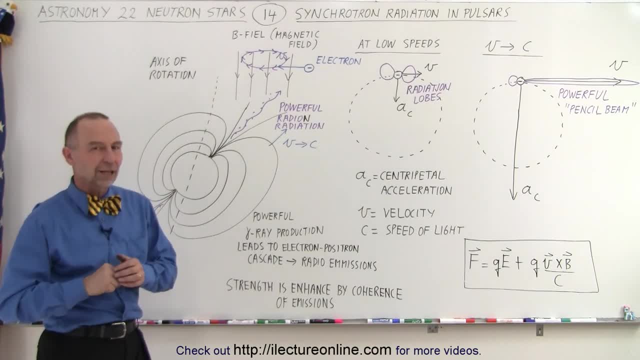 It's the charges that are being shot out near the speed of light that produce the electromagnetic radiation. Hence the pulsar, Hence the pulsar, Yep, that's it. Yeah, without those fast-moving charges like this, there's an electron electron like that. 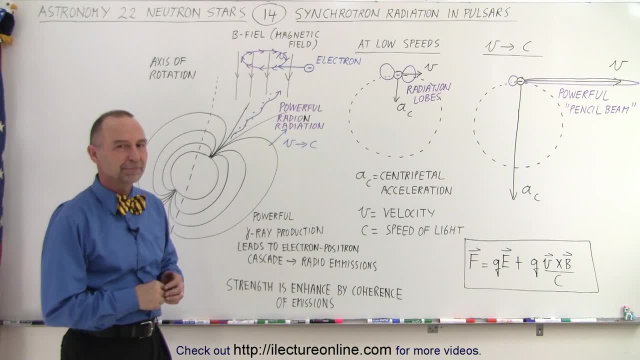 you wouldn't see those. the radiation: I don't understand about the radiation loads. Well, when you have charges move around in circles, you have radiation. The radiation goes along the path of the direction of the velocity of the electrons. The faster you move, the narrower and the more powerful.